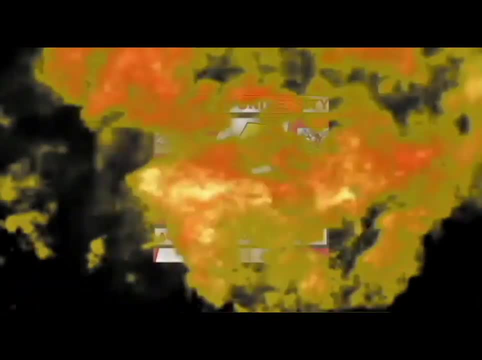 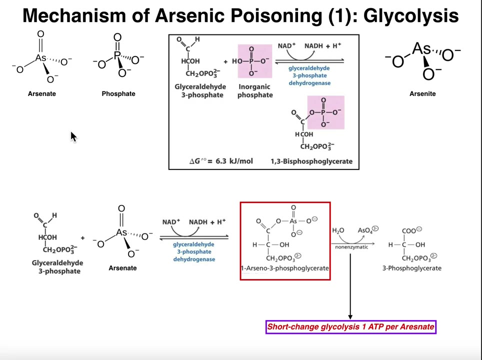 Welcome back to Catalyst University. My name is Kevin Tokoff. Please make sure to like this video and subscribe to my channel for future videos and notifications. In this video, we're going to talk about the mechanism of arsenic poisoning, And actually there's a lot of. 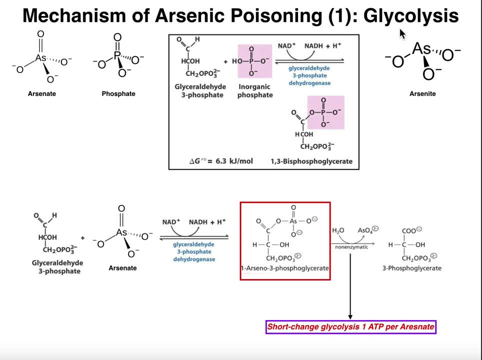 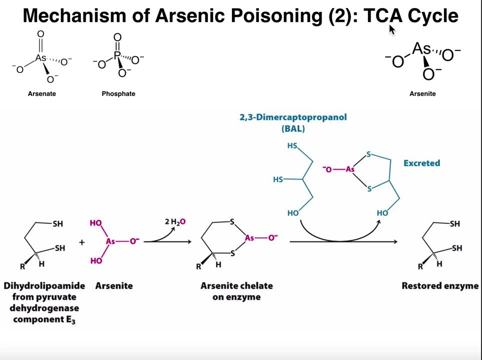 different mechanisms, but we're going to look at two. The first one is a very minor one. This is actually how arsenic actually disrupts glycolysis, but there's a major mechanism of arsenic poisoning and that's the disruption of the TCA cycle. So we'll actually look at that. First, let's look. 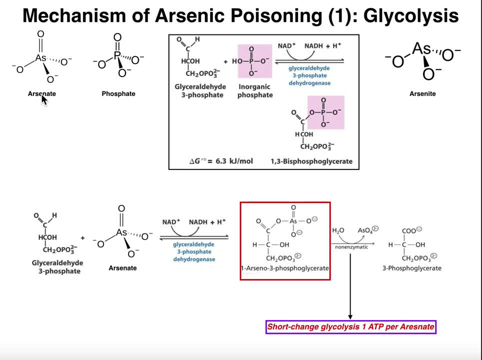 at a couple of things about the form of arsenic. The two most common forms of arsenic are arsenate and arsenite. Now arsenate: if you look at its chemical structure other than the central atom of arsenic, it's going to resemble the molecule of phosphate very closely- Again, the central atom. 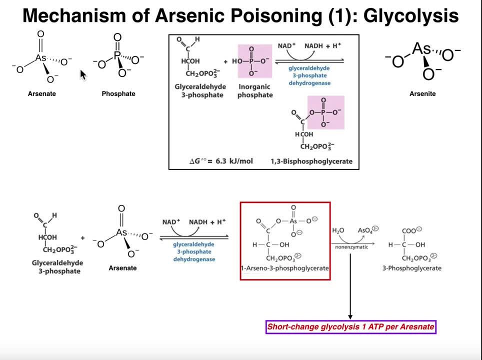 is different, but we still have four oxygens and a net charge of minus three on the molecule. Arsenite is a more reduced form of the arsenic, but again it still has three negative charges. It turns out that the arsenite is going to be important in, or I should say deadly in, the TCA. 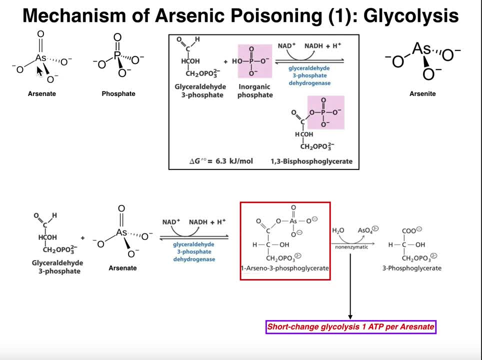 cycle, whereas this form of arsenic, the arsenate, is going to be the one that disrupts glycolysis. So let's first talk about the glycolytic reaction that is most deleteriously affected, And that is the enzyme glyceraldehyde 3-phosphate dehydrogenase. This enzyme, I believe, is number. 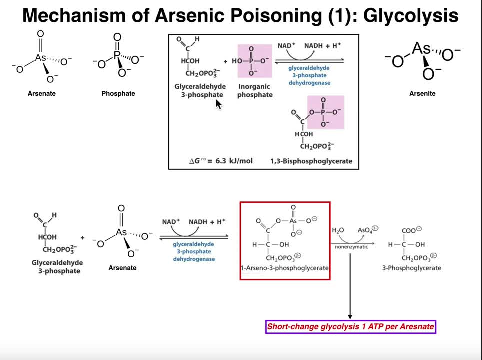 six. in the pathway It converts glyceraldehyde 3-phosphate with an inorganic phosphate into 1,3-bisphosphoglycerate. Notice what it's doing. It's actually taking using an oxidation with NAD, but it's taking this phosphate right here and essentially swapping it with this hydrogen on. 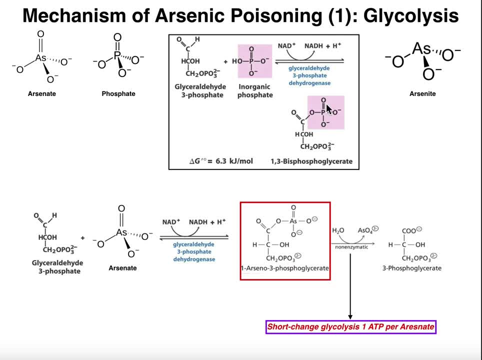 this carbon. So this carbon will no longer have a hydrogen. it'll actually have this phosphate, And what this 1,3-bisphosphoglycerate is going to allow is net ATP generation through the payoff phase of glycolysis. So it turns out that, from the perspective of this enzyme, 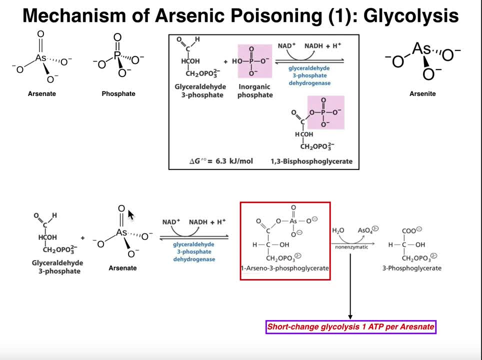 the enzyme can't really distinguish well between phosphate and arsenate because they are so chemically similar. So instead of adding phosphate, if we've got a lot of arsenate floating around the cytoplasm, which is where glycolysis occurs, this enzyme- the same enzyme up here- can actually add. 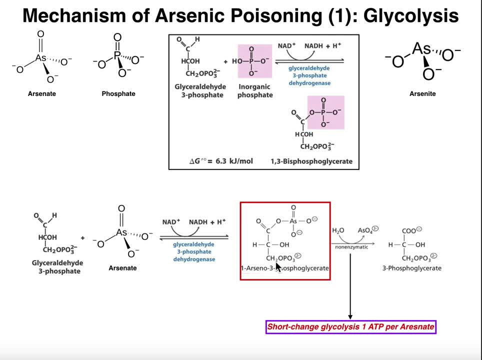 phosphate to this enzyme, And so what you'll end up with is this molecule, which is called 1-arsenal-3-phosphoglycerate, which looks almost identical to 1,3-bisphosphoglycerate, except for this phosphate is now replaced by an. 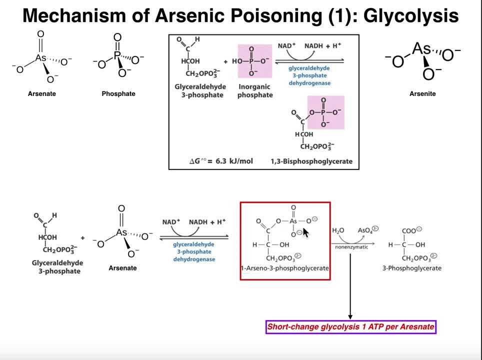 arsenate. Now, obviously you cannot make ATP from this And in any case, what will happen is you'll have a non-enzymatic hydrolysis where water will actually come and knock off this arsenate Again, generate more arsenate, which can then go back and do the same reaction again. This arsenate can go. 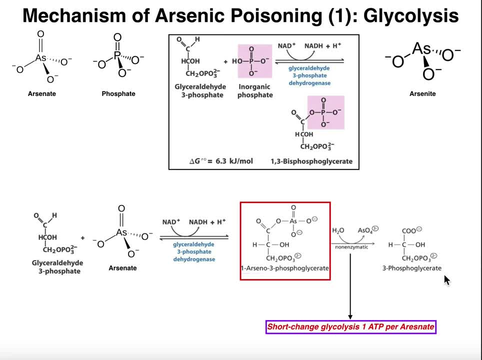 back over here. But what also happens is you get 3-phosphoglycerate Normally in glycolysis. what will happen after you generate 1,3-bisphosphoglycerate is you'll have the enzyme phosphoglycerate kinase. Phosphoglycerate kinase will actually convert 1,3-bisphosphoglycerate. 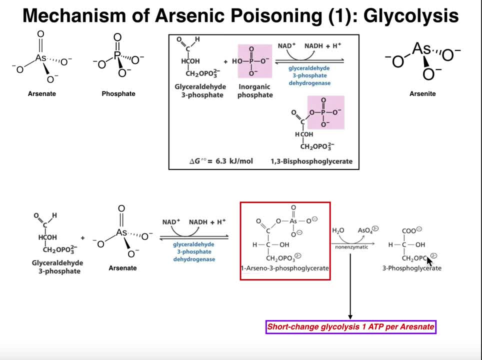 into 3-phosphoglycerate, but it will generate an ATP in the process And you can go back to glycolysis and look at that. By having this non-enzymatic hydrolysis, we get directly to 3-phosphoglycerate, And so what happens is is for every molecule of arsenate that 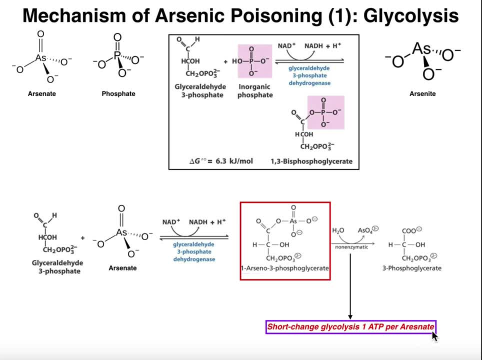 enters this, we shortchange glycolysis 1 ATP. So again, this is really bad because due to this non-enzymatic hydrolysis, this arsenate can then go back and react again with glyceraldehyde 3-phosphate to form more of this compound. 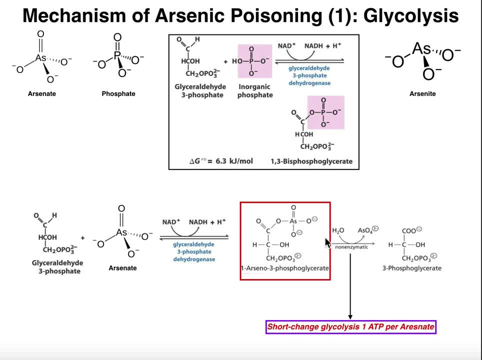 In glycolysis. this is not completely toxic. I mean, it's certainly not good, It's not really lethal, It's just going to shortchange your energy. But the kicker is how arsenic actually disrupts the TCA cycle and this is really bad. So here we have the enzyme. 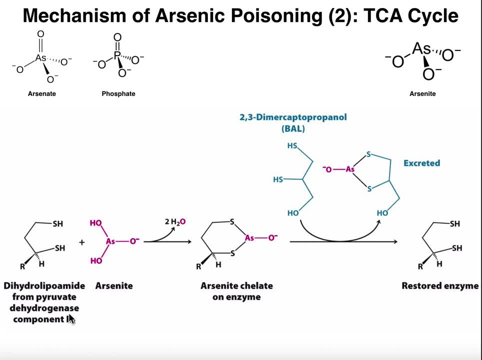 pyruvate dehydrogenase. This is actually the enzyme 3 or E3 component of it, And the same thing can actually happen to the alpha-ketoglutarate dehydrogenase enzyme in the TCA cycle. This is the cofactor. 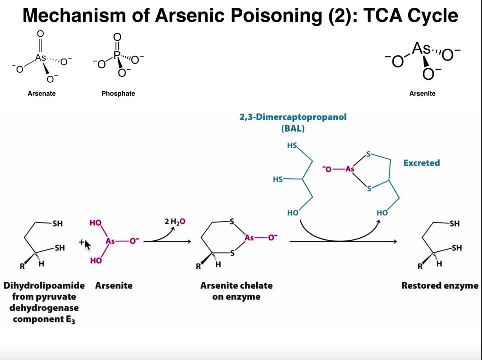 At least part of it- dihydrolipoamide. This is normally going to be involved in binding one of the binding, the acetyl group, and then transferring it to coenzyme A, But what can happen is these two thiol groups can actually attack this arsenic atom right here. Okay, 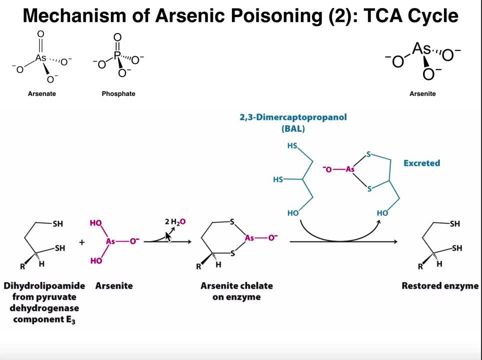 when they attack this atom, these two OHs are lost as two waters, And what you have now is this dihydrolipoamide: the sulfur here bound to this arsenic and the sulfur here bound to the same arsenic Again. this oxygen here is still there. This is really bad, This. 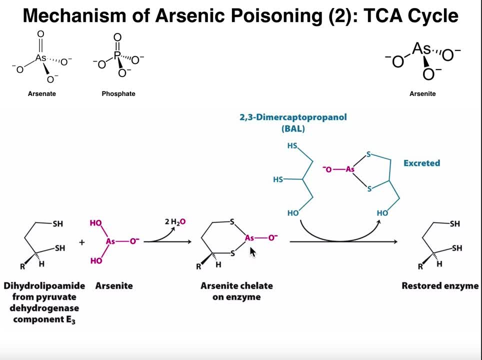 is called the arsenate chelate on the enzyme Arsenic. even though it's a metalloid, technically, it's behaving here more as a metal, And so what we say is that this arsenic is actually chelated to the enzyme and it's a very, very strong interaction. This isn't going anywhere. 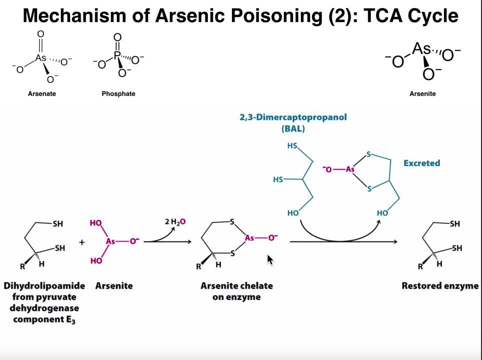 So more or less you could consider this suicide inhibition, because this is not coming off and it basically kills the enzyme's activity And really by killing the TCA cycle, if you have enough of this arsenate, you basically kill metabolism. Now, if you actually catch, 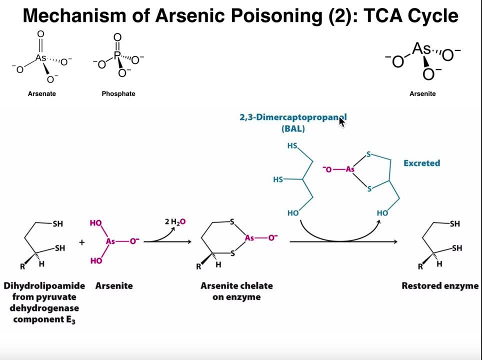 this poisoning early on, you can add a drug. This is actually an antidote called 2,3-dimercaptopropanol, and I'm not sure why it's called BAL, but that's the abbreviation for it, And it's this. 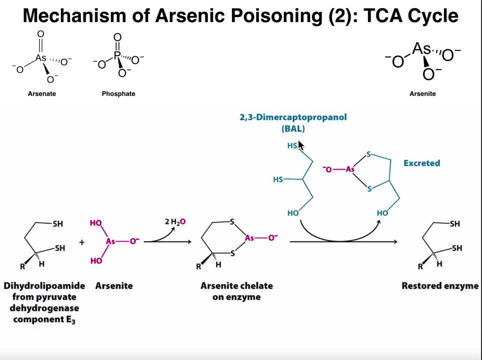 molecule right here in blue. What this molecule can then do, once you already have this arsenic chelated on here, is these two sulfurs can actually compete for the arsenic, So what they'll do is they actually will have a stronger interaction with the arsenic than these two. on the dihydrolipoamide. 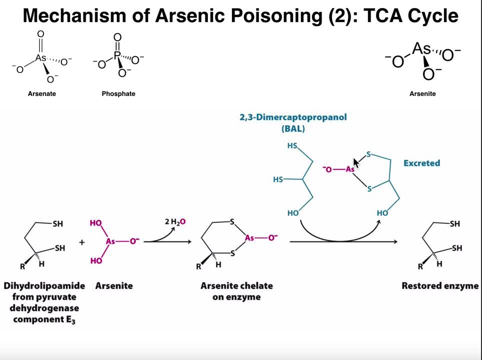 And so these two sulfurs will then bind the arsenic. as you see right here and now we have a restored enzyme, So that's how the antidote works. Additionally, notice this arsenic also still has this oxygen with a negative charge, and you also have an OH group on here, which 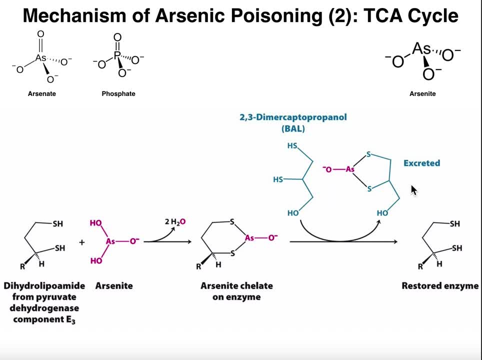 is polar, So you have over here a polar charged molecule which can easily then be excreted. So that's how this 2,3-dimercaptopropanol is going to act as an antidote for arsenite poisoning.